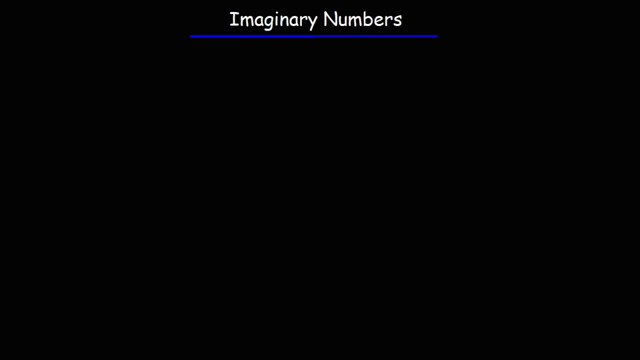 In this video we're going to talk about imaginary numbers. Imaginary numbers are basically complex numbers with the imaginary unit I, I is equal to the square root of negative 1.. I squared is negative 1. And I to the third is equal to negative I. I to the fourth is equal to. 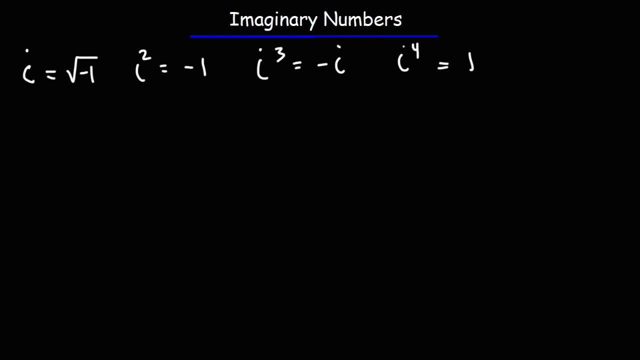 1.. Now let's talk about why that's the case, Starting with I to the third power. You can think of I to the third power as I squared times I, And since I to the second power is negative, 1, I to the third reduces to negative I In the case of I to the fourth. think of: 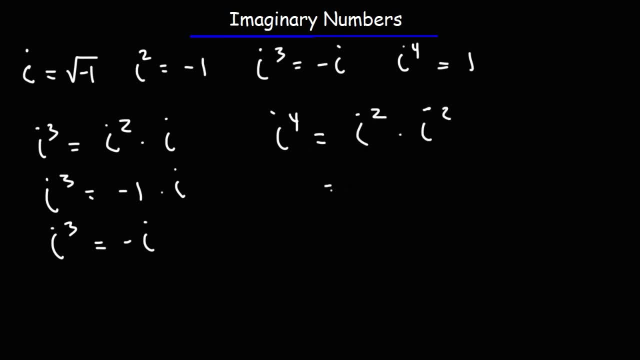 it as I squared times I squared, So it's negative 1 times negative 1.. And since I to the third is positive 1, which is positive 1.. So, with that in mind, how would you simplify these imaginary numbers? Let's say, if you have I to the seventh power, I to the twenty-sixth. 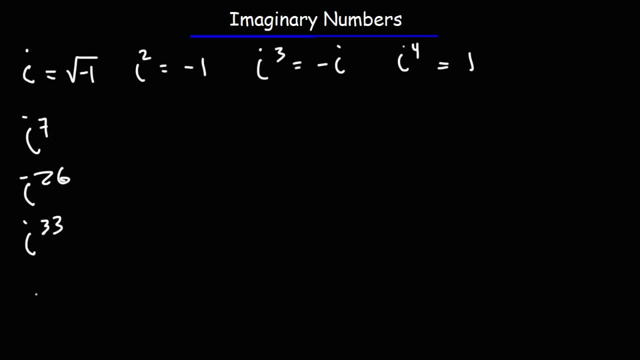 power, I to the thirty-third power and I to the forty-third power. Go ahead and try these. What I would recommend doing is breaking up each exponent using the highest multiple of four. So I to the seventh. you can break it up as I to the fourth times, I to the third, I to 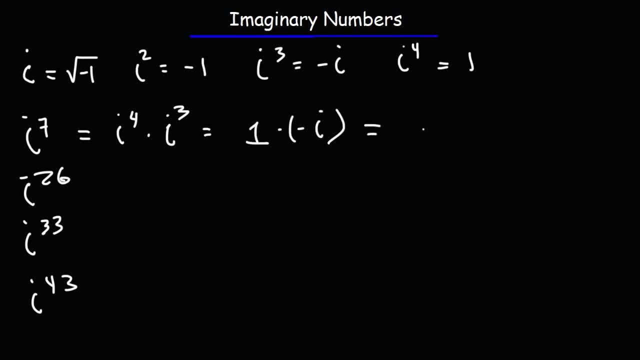 the fourth is 1.. I to the third is negative I. So I to the seventh reduces to negative I. Now let's move on to the next one. I raised to the twenty-sixth power. So what is the highest multiple of four? just under twenty-sixth. Well, twenty-four is a multiple of four. So 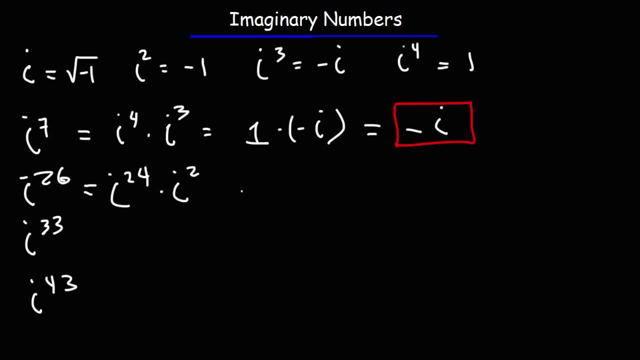 what I would do is I would write it as I to the fourth times I to the twenty-sixth power, I to the twenty-four times. I squared Now, I to the twenty-four is basically four times six, So it's I to the fourth raised to the sixth power. I to the fourth is 1.. If you 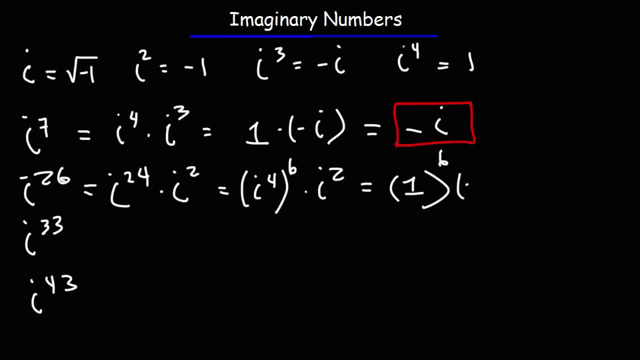 raise 1 to the sixth power, it's still going to be 1. And we can replace I squared of negative 1.. So thus I to the twenty-sixth can be reduced to negative 1.. Now let's move on to the next. 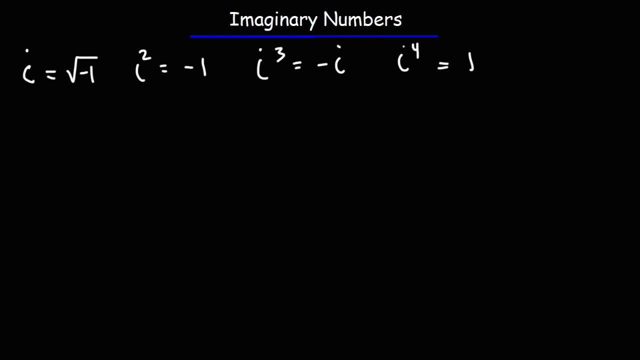 1.. Now let's talk about why that's the case, Starting with i to the third power. You can think of i to the third power as i squared times i, And since i to the second power is negative, 1, i to the third reduces to negative i In the case of i to the fourth. think of: 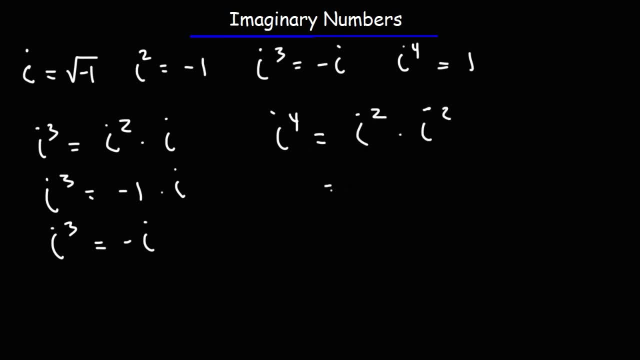 it as i squared times i squared, So it's negative 1 times negative 1.. And since i to the third is positive 1, which is positive 1.. So, with that in mind, how would you simplify these imaginary numbers? Let's say, if you have i to the seventh power, i to the twenty-sixth. 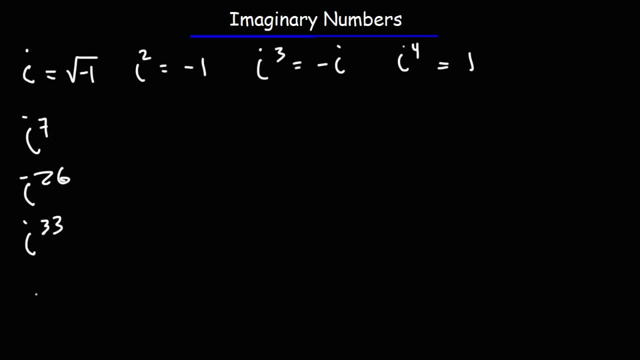 power, i to the thirty-third power and i to the forty-third power. Go ahead and try these. What I would recommend doing is breaking up each exponent using the highest multiple of four. So i to the seventh. you can break it up as i to the fourth times, i to the third, i to 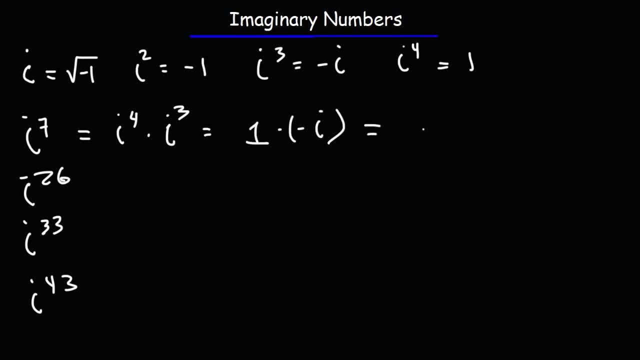 the fourth is 1.. i to the third is negative i. So i to the seventh reduces to negative i. Now let's move on to the next one. i raised to the twenty-sixth power. So what is the highest multiple of four? just under twenty-sixth. Well, twenty-four is a multiple of four. So 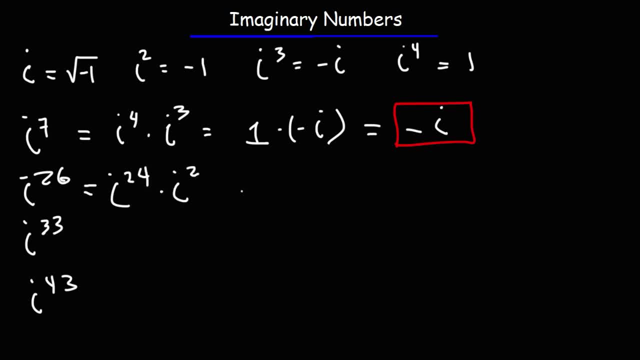 what I would do is I would write it as i to the fourth times i to the twenty-sixth power. So i to the fourth is 1.. Now, i to the twenty-four is basically 4 times 6.. So it's i to the fourth. 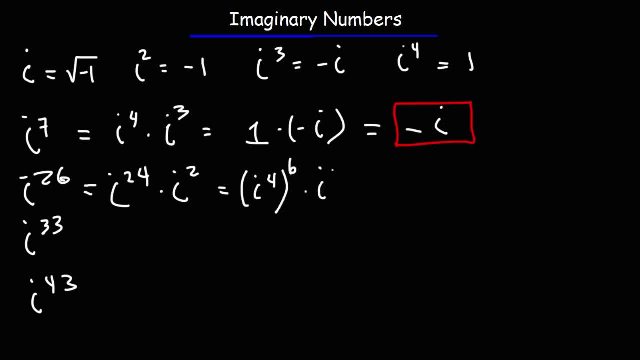 raised to the sixth power. i to the fourth is 1.. If you raise 1 to the sixth power, it's still going to be 1. And we can replace i squared of negative 1.. So thus, i to the twenty-sixth. 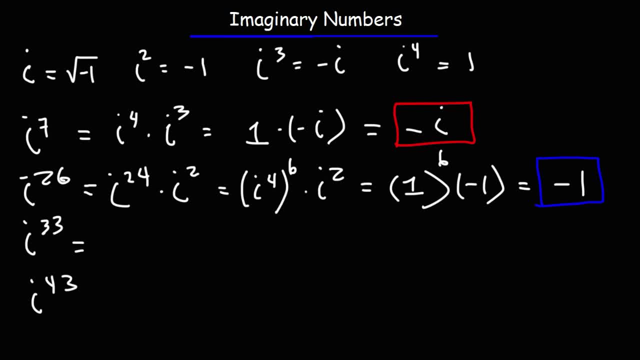 can be reduced to negative 1.. Now let's move on to the next one, i to the thirty-third power. The highest multiple of 4, just under 33, is 32.. So we can break up 33 as 32 plus 1.. And 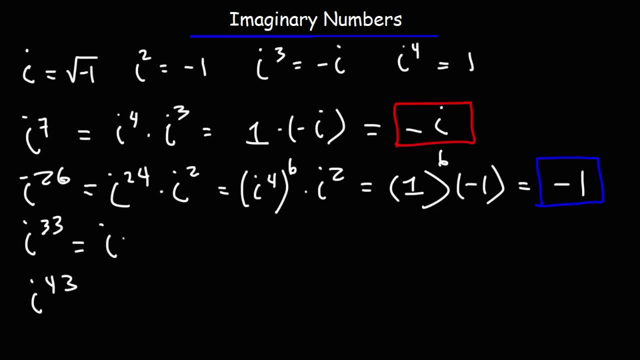 one: I to the thirty-third power. The highest multiple of four, just under thirty-three, is thirty-two. So we can break up thirty-three as thirty-two plus one, And thirty-two is four times eight. So this is going to be one raised to the eighth power, times I, which is simply I. Now for the last one: I to the 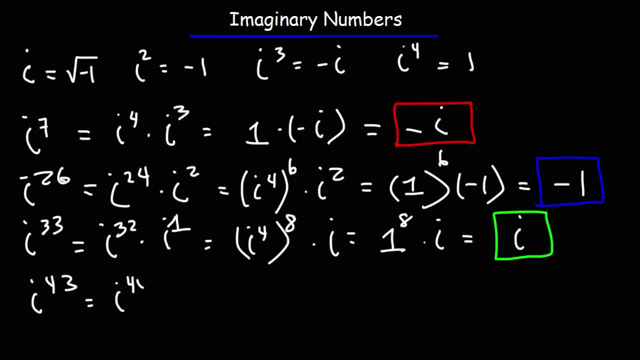 forty-third power. We can break it up to I to the forty-third power, So this is going to be I to the forty times. I cubed I to the forty. I'm going to write as I to the fourth raised to the tenth power And I to the third is negative I, So we can replace I to the. 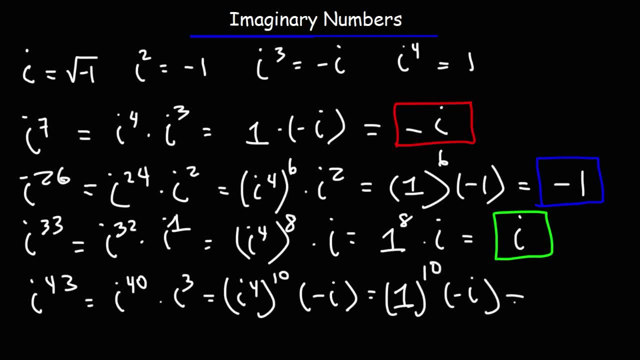 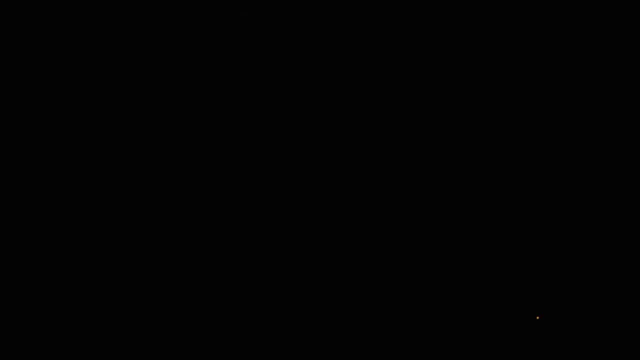 fourth with 1.. And so the final answer is just going to be negative. I So that's how you could simplify imaginary numbers with very large exponents. Now let's talk about adding and subtracting imaginary numbers. So let's say you have this: 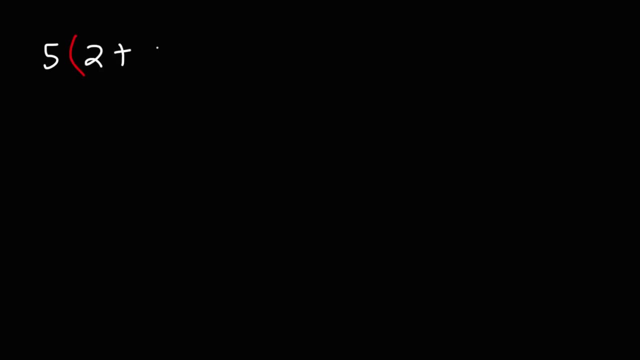 problem: Times two plus three, I, Let's say minus four. And then times seven minus two, I. How would you simplify this expression? Feel free to try this problem if you want to. In order to simplify this expression, the first thing we need to do is distribute. Let's distribute. 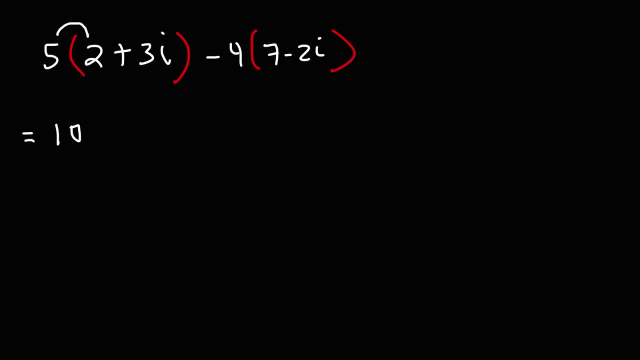 five to two plus three: I. Five times two is ten. Five times three, I is fifteen. And then five times three is fifteen: I. Negative. four times seven is negative. twenty-eight Negative. four times negative two: I is positive, eight, I. Now, at this point we need to combine like: 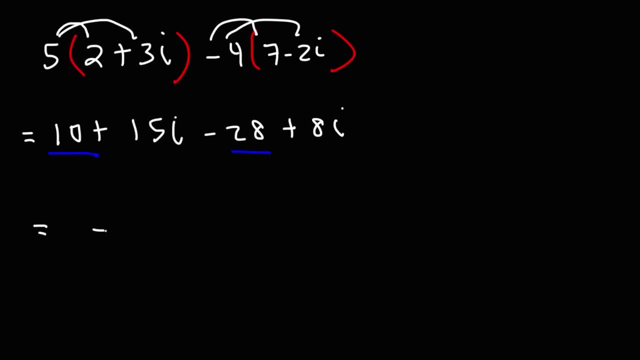 terms. So we can combine ten and negative twenty-eight: That's negative eighteen, And then fifteen I and eight I, That's going to be positive twenty-three I. So at this point our answer is in standard form: A plus B I. A is the real part of the complex. 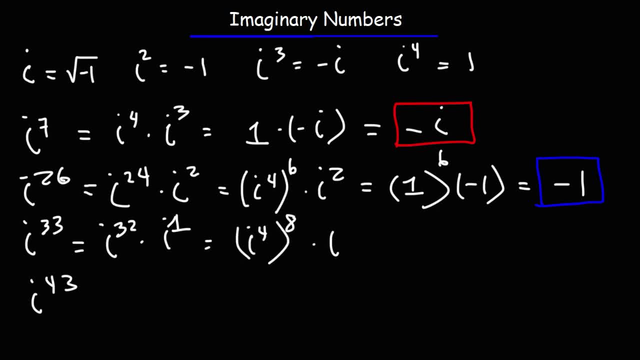 32 is 4 times 8.. So this is going to be 1 raised to the eighth power times i, which is simply i. Now for the last one, i to the forty-third power. we can break it up to i to the forty times. i cubed i to the forty. I'm going to write as i to the fourth raised. 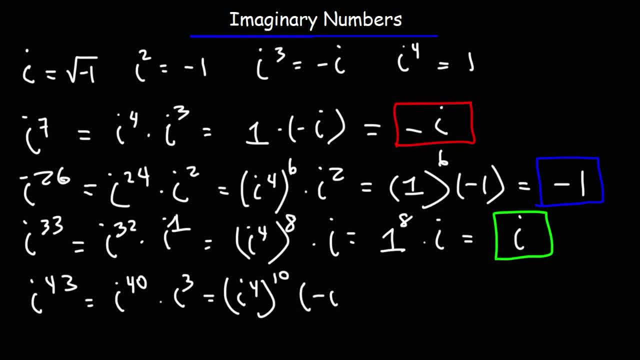 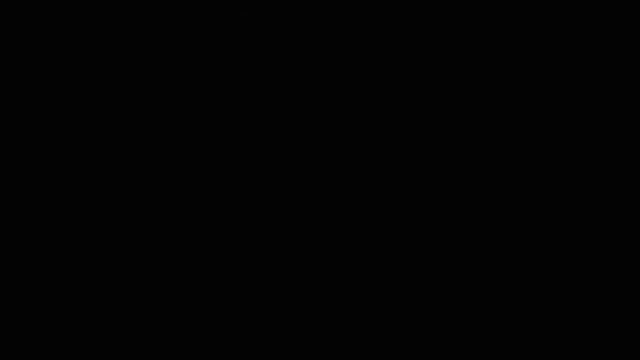 to the tenth power And i to the third is negative i. So we can replace i to the fourth with 1.. And so the final answer is just going to be negative i. So that's how you could simplify imaginary numbers with very large exponents. 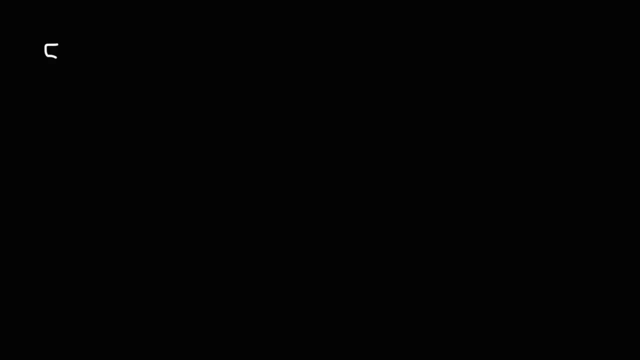 Now let's talk about adding and subtracting imaginary numbers. So let's say you have this problem. Let's say i to the fourth, raised to the tenth power, times 2 plus 3i- let's say minus 4, and then times 7 minus 2i. How would you simplify this expression? Feel free to try this problem. 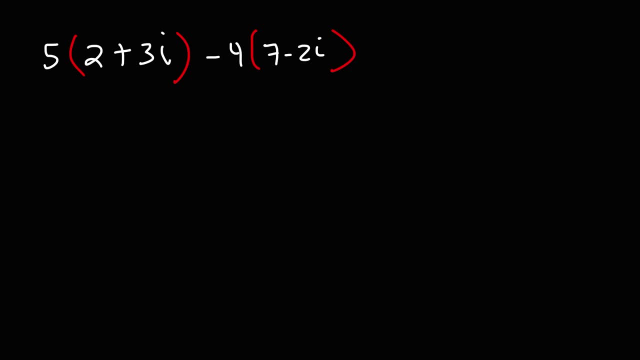 if you want to. In order to simplify this expression, the first thing we need to do is distribute. Let's distribute 5 to 2 plus 3i. 5 times 2 is 10.. 5 times 3i is 15.. 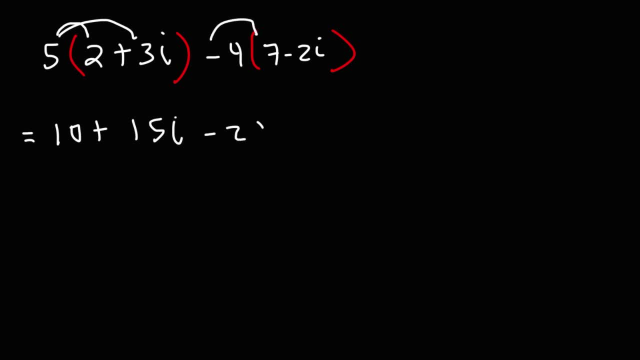 Negative 4 times 7 is negative 28.. Negative 4 times negative 2i is positive 8i. Now, at this point we need to combine like terms. So we can combine 10 and negative 28, that's negative 18.. And then 15i and 8i, that's going to be positive 23i. 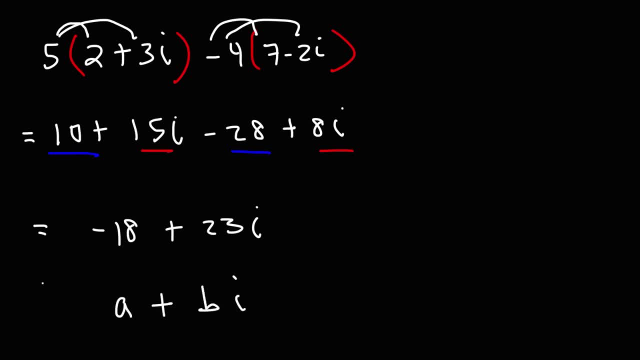 So at this point our answer is, in standard form: a plus bi. a is the real part of the complex. This is a real number, so is b, But combined this makes up the imaginary part b times i, Even though b is a real number, but combined b times i is an imaginary number. 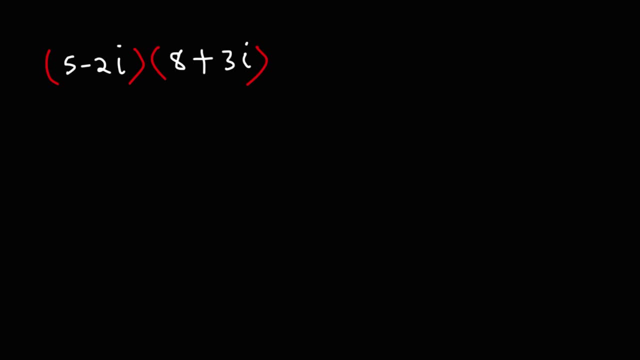 So that's the solution for this particular problem. Now let's work on this example. So here we're going to multiply two imaginary numbers together. So we need to FOIL: 5 times 8 is 40.. 5 times 3i, that's going to be 15i. 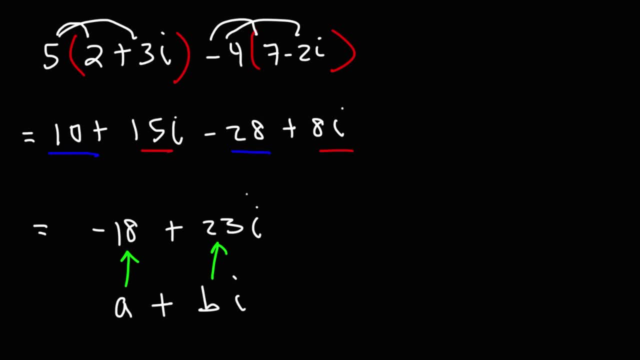 number. So is B, But combined this makes up the imaginary part B times I, Even though B is the real number, But combined B times I is an imaginary number. So that's the solution for this particular problem. Now let's work on this example. So here we're going to multiply. 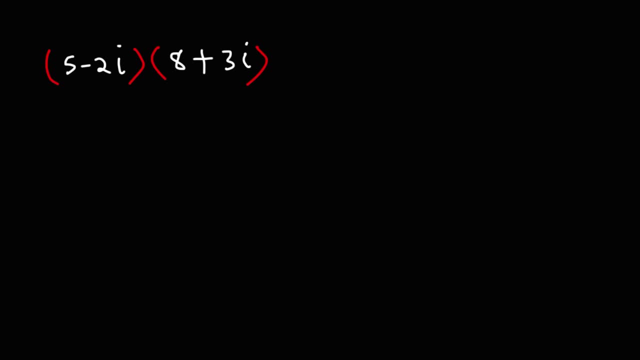 two imaginary numbers together. So we need to FOIL: Five times eight is forty, And then five times three I, That's going to be fifteen I, And then negative two. I times eight, That's negative sixteen I, And then negative two. I times three I, That's negative six, I squared. 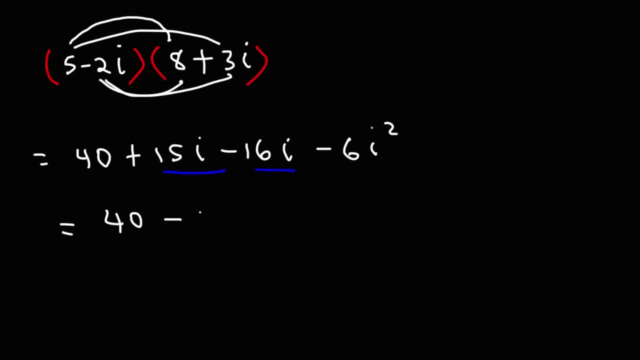 So all we can do right now is combine like terms And then simplify: Now I squared is negative one, So six negative six, I squared is going to be positive six, And now we can combine these two And so we're going to get forty-six. 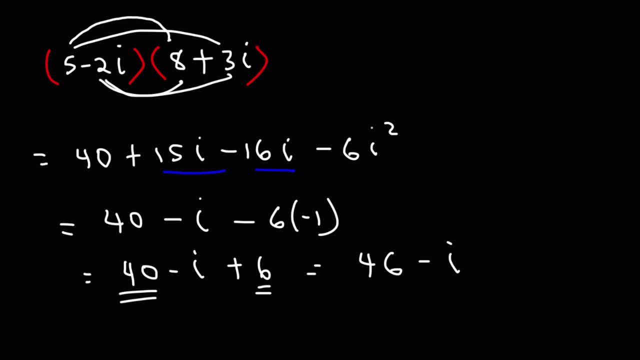 minus I. So when simplifying imaginary numbers, or if you're multiplying or dividing, you always want to put your final answer in standard form: A plus B, I form. So in this example, A is forty-six, B is the number in front of I, which is negative one. So you can write: 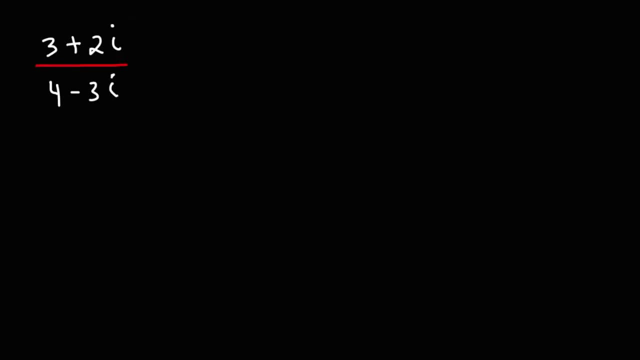 it as forty-six minus one I. if you want. Now let's try this one. How can we simplify this expression? Three plus two, I divided by four minus minus 3i. So what do we need to do here When dividing complex numbers? one of the best things. 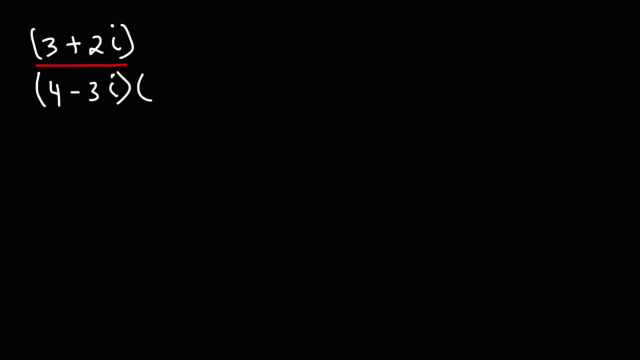 to do is to multiply the denominator by the conjugate of the complex number. So the conjugate of 4 minus 3i is simply 4 plus 3i. You just need to change a sign between the real and imaginary number. Now, whatever you do to the bottom, you must also do to the top. So we got to multiply. 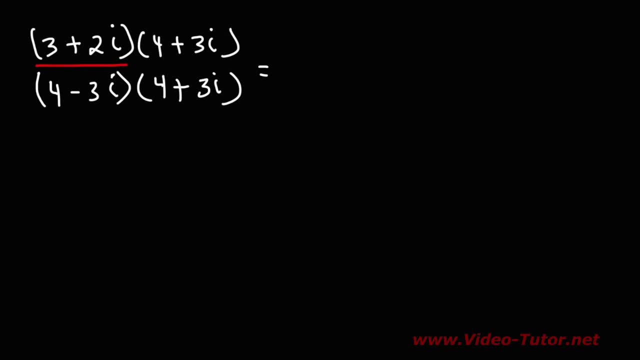 both the numerator and the denominator by the conjugate of the denominator. Now we need to FOIL 3 times 4 is 12.. 3 times 3i, that's going to be 9i, And then 2i times 4,. 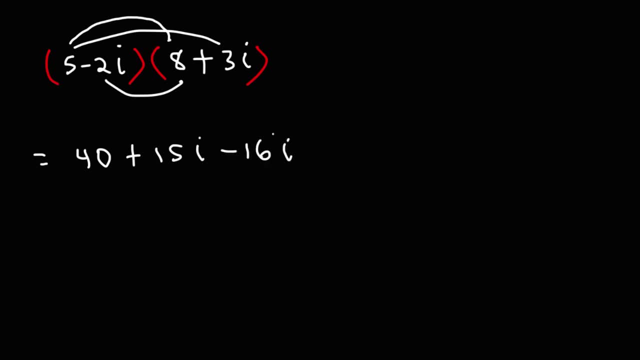 And then negative 2i times 8,, that's negative 16i. And then negative 2i times 3i, that's negative 6i squared. So all we can do right now is combine like terms and then simplify. 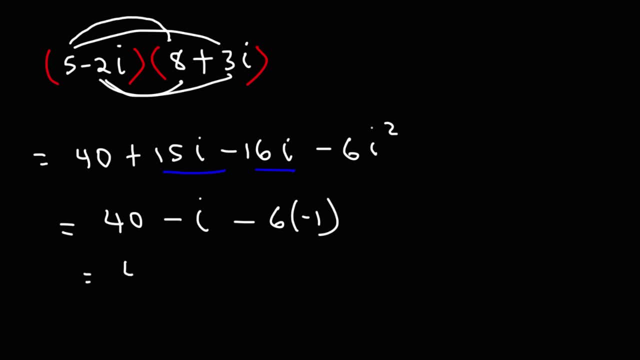 Now i squared is negative 1.. So 6, negative 6i squared is going to be positive 6. And now we can combine these two, And so we're going to get 46 minus i. So when simplifying imaginary numbers, or if you're multiplying or dividing, you always 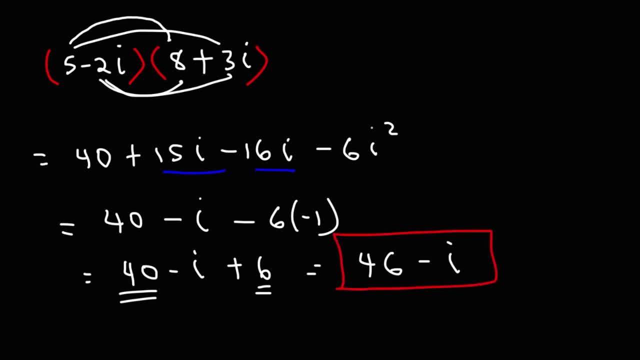 want to put your final answer in standard form, a plus bi form. So in this example, a is 46, b is the number in front of i, which is negative 1. So you can write it as 46 minus 1i if you want. 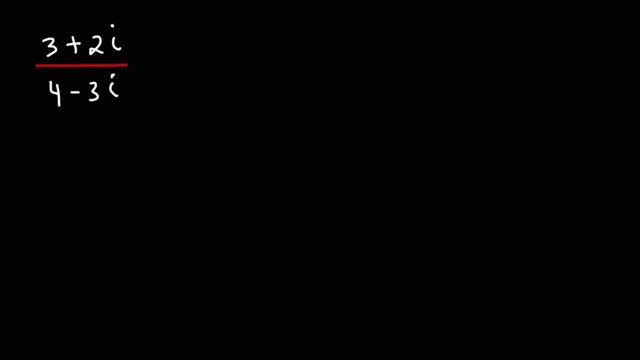 Now let's try this one. How can we simplify this expression: 3 plus 2i Divided by 4 minus 3i. So what do we need to do here? When dividing complex numbers, one of the best things to do is to multiply the denominator. 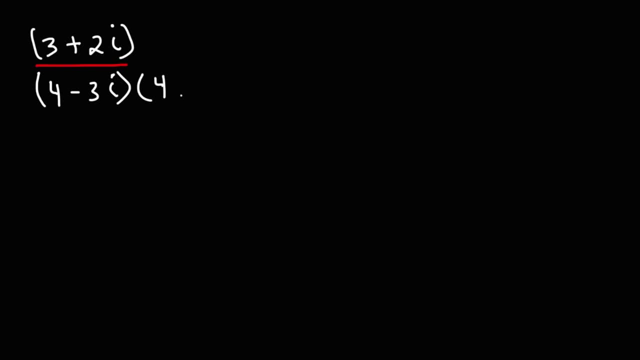 by the conjugate of the complex number. So the conjugate of 4 minus 3i is simply 4 plus 3i. You just need to change a sign between the real and the imaginary number. Now, whatever you do to the bottom, you must also do to the top. 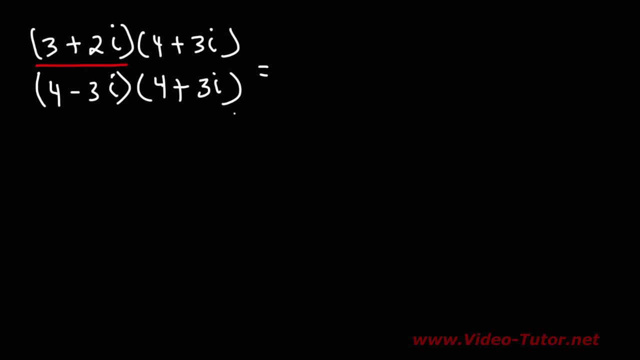 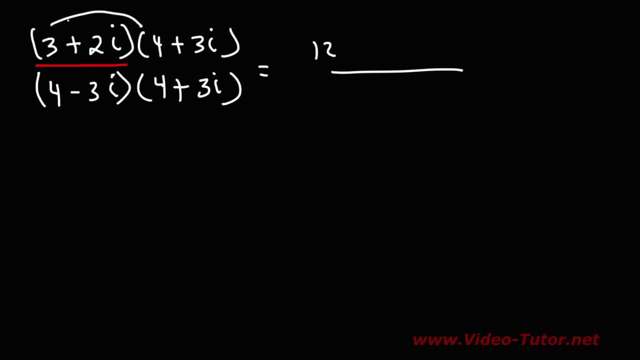 denominator. Now we need to FOIL: 3 times 4 is 12.. 3 times 3i, that's going to be 9i, And then 2i times 4, that's 8i. 2i times 3i, that's going to be plus 6i squared. 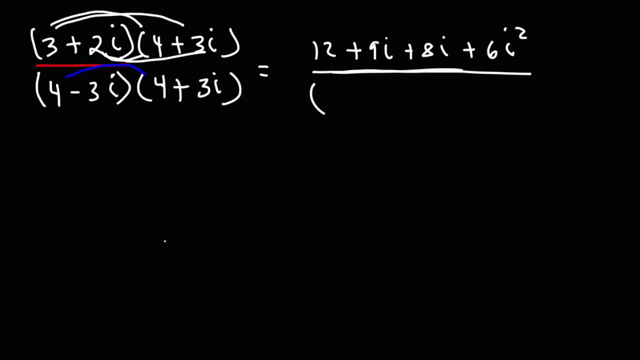 On the bottom we have 4 times 4, which is 16.. Well, we can get rid of the parentheses. We can do it again. So i times 3i, that's going to be plus 6i squared. 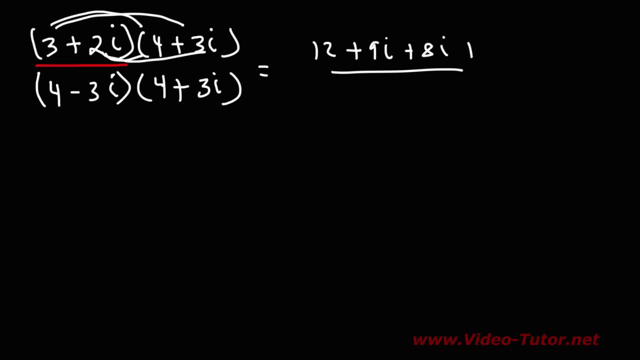 that's 8i. 2i times 3i, that's going to be plus 6i. squared On the bottom, we have 4 times 4, which is 16.. well, we can get rid of the parentheses. next is going to be 4 times 3i. 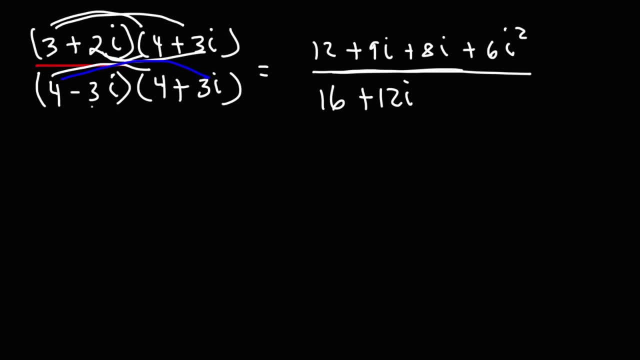 that's going to be plus 12i and that's going to cancel with negative 3i times 4, which is negative 12i, and then negative 3i times positive 3i, that's negative 9i squared. so now let's simplify. 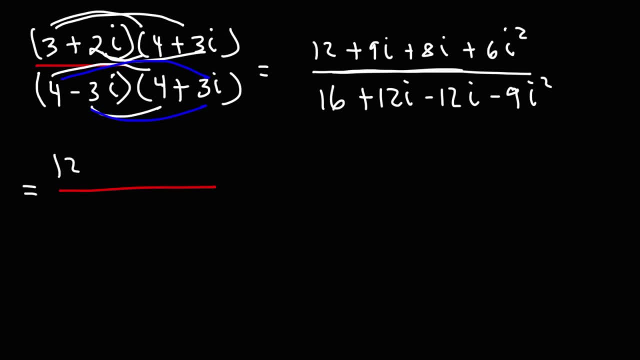 9i plus 8i is 17i and 6i squared is negative 6. these two will cancel negative 9i squared. i squared is negative 1, so negative 9i squared is going to be plus 9. on top we can combine 12 minus 6. 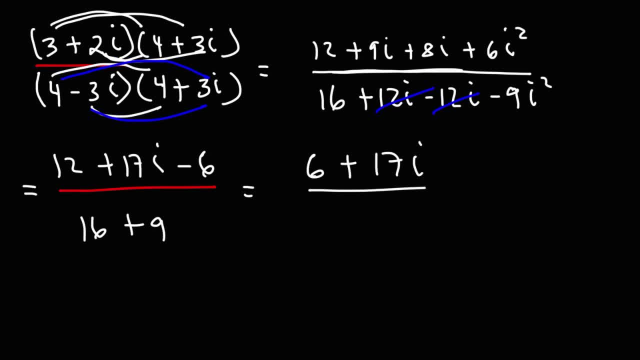 which is 6, and on the bottom, 16 plus 9 is 25. so now let's simplify. so right now we can write the answer as 6 over 25 plus 7. i mean 17 over 25 times i. so this is the solution in standard form. 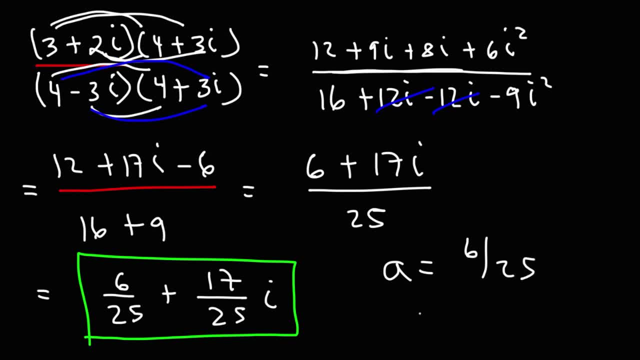 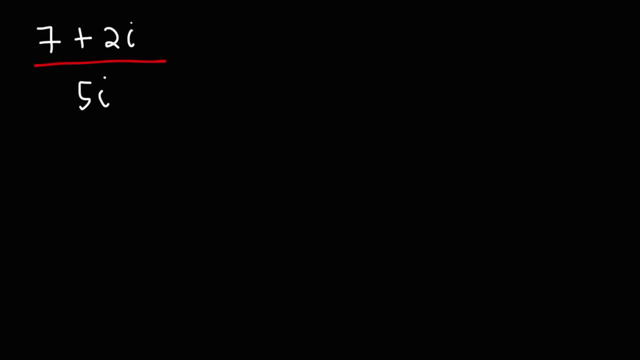 so we can see that a is 6 over 25. b is 17 over 25. now what would you do if you were to see a problem like this? how would you simplify this problem? notice that we don't have an a value in the denominator. 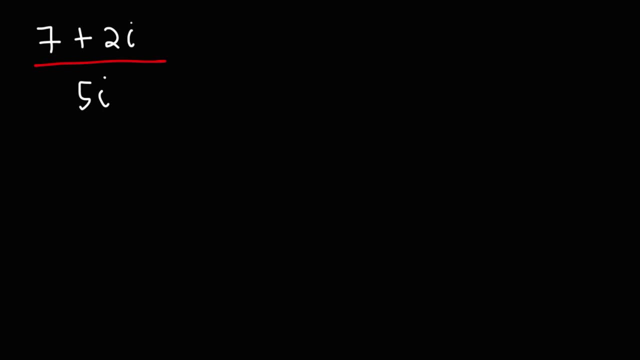 of the fraction. we only have the b value attached to i. in a situation like this, the best thing to do is to multiply the top and the bottom by i 7 times. i is 7i. 2i times i is going to be 2i squared. 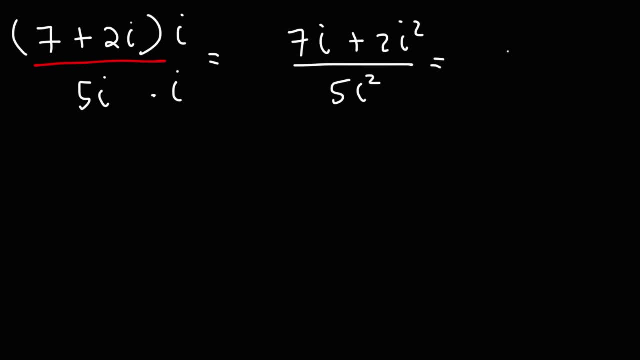 on the bottom we're going to have 5i squared, now 2i squared. that can be rewritten as negative 2. 5i squared is negative 5, so now we can put it in standard form. so we have negative 2 divided by 9. 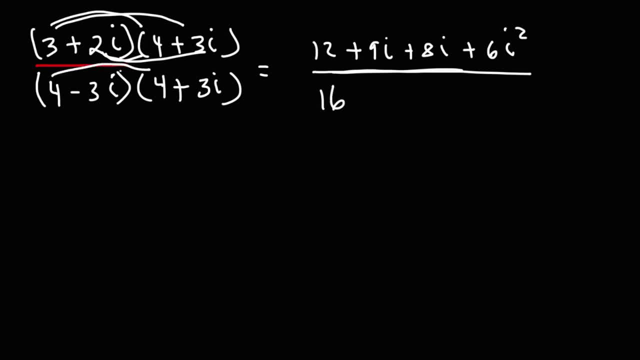 On the bottom we have 4 times 4, which is 16.. next is going to be 4 times 3i, that's going to be plus 12i and that's going to cancel with negative 3i times 4, which is negative 12i, and then negative 3i times positive 3i. 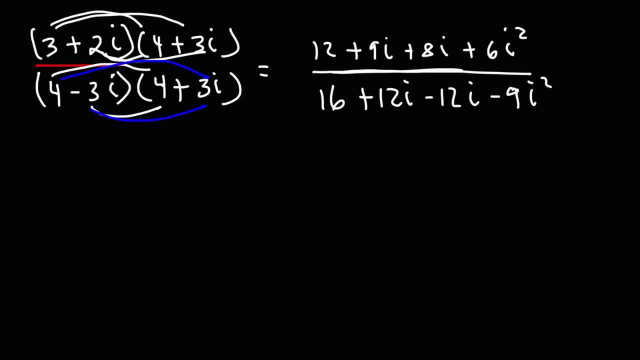 that's negative 9i squared. So now let's simplify: 9i plus 8i is 17i and 6i squared is negative 6. These two will cancel Negative 9i squared. i squared is negative 1, so negative 9i squared is going to be plus 9.. 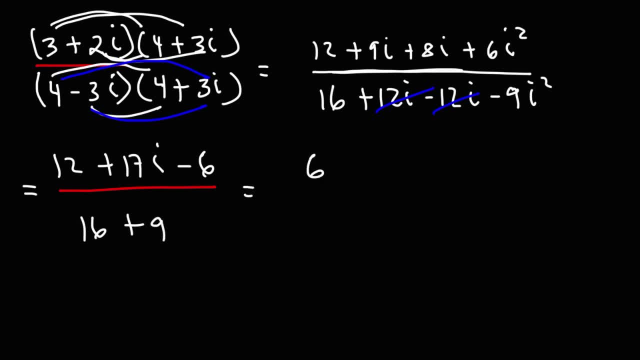 On top we can combine 12 minus 6,, which is 6,, and on the bottom, 16 plus 9 is 25.. So right now we can write the answer as 6 over 25 plus 7,, I mean 17 over 25 times i. 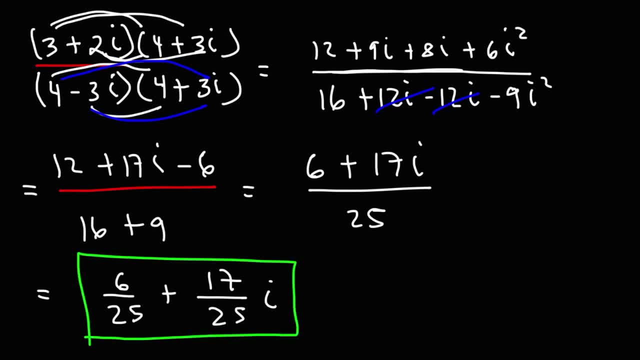 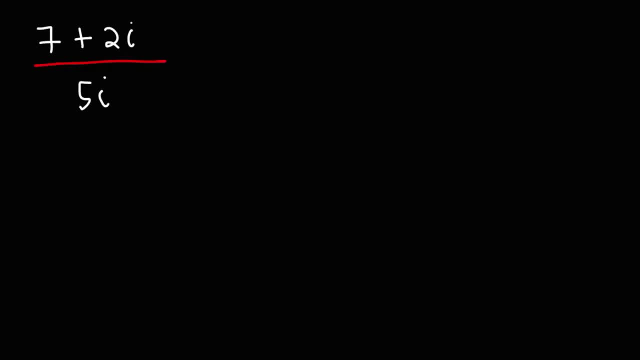 So this is the solution in standard form. So we can see that a is 6 over 25,, b is 17 over 25.. Now what would you do if you were to see a problem like this? How would you simplify this problem? 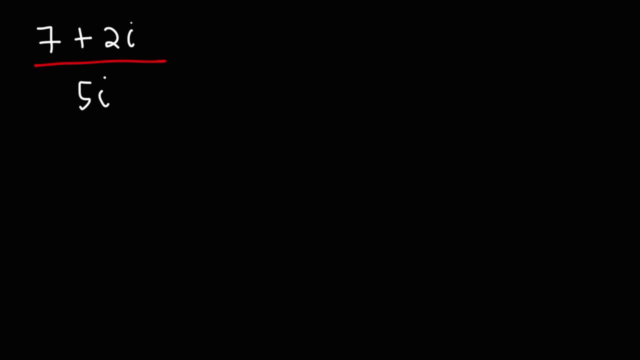 Notice that we don't have an a value in the denominator of the fraction. We only have the b value attached to i. In a situation like this, the best thing to do is to multiply the top and the bottom by i 7 times i is 7i. 2i times i is going to be 2i. squared On the bottom, we're going to have 5i. 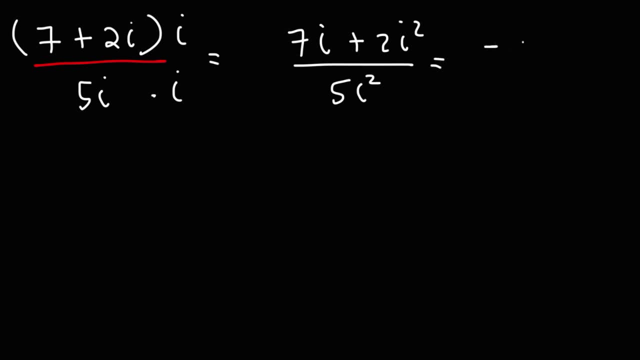 squared, Now 2i squared. that can be rewritten as negative 2.. 5i squared is negative 5.. So now we can put it in standard form. So we have negative 2 divided by negative 5, which is positive 2 over 5, and then positive 7i over negative 5,, that's negative. 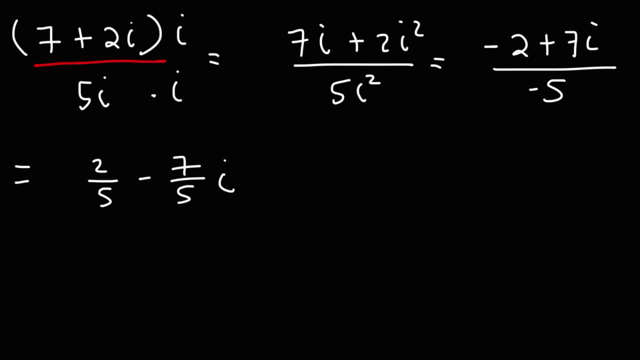 7 over 5i. So now we have our answer in a plus bi form: a is 2 over 5,, b is negative, 7 over 5.. So you always want to simplify your answer to standard form. Now, sometimes you may need to solve equations associated with complex numbers. 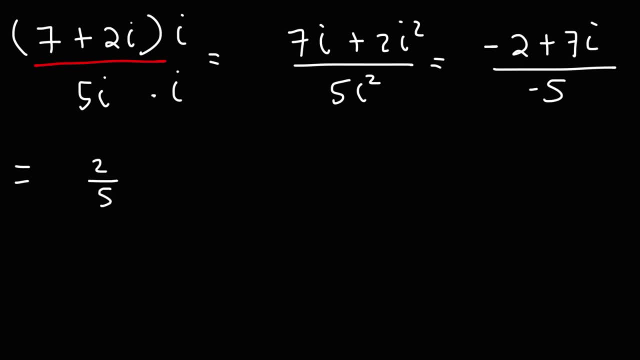 i minus negative 5, which is positive 2 over 5, and then positive 7i over negative 5, that's a negative 7 over 5i. so now we have our answer in a plus bi form. a is 2 over 5. 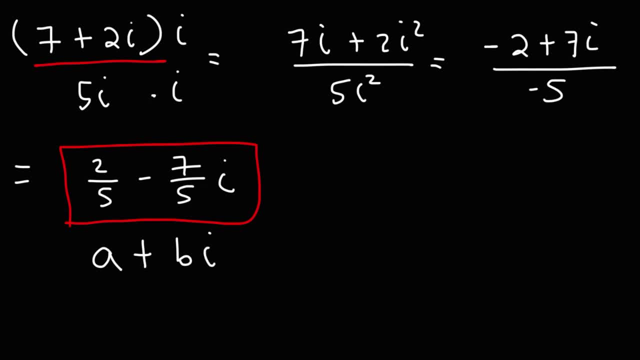 b is negative, 7 over 5. so you always want to simplify your answer to standard form. now, sometimes you may need to solve equations associated with complex numbers. so let's say we look at different numbers and you might be trying to solve one of different kinds of equations. 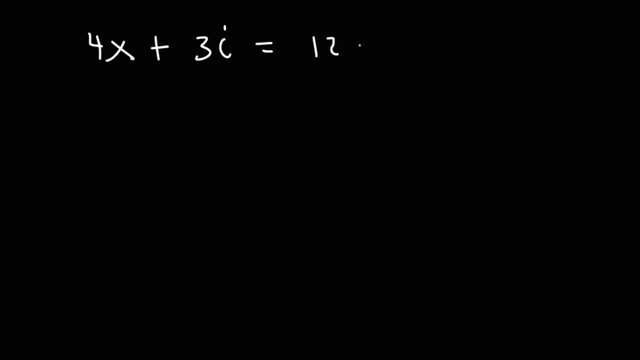 So let's say we have the equation: 4x plus 3i is equal to 12 minus 15y times i. So what is the value of x and y in this equation? In order to solve this equation, we need to identify the real portion of the complex number. 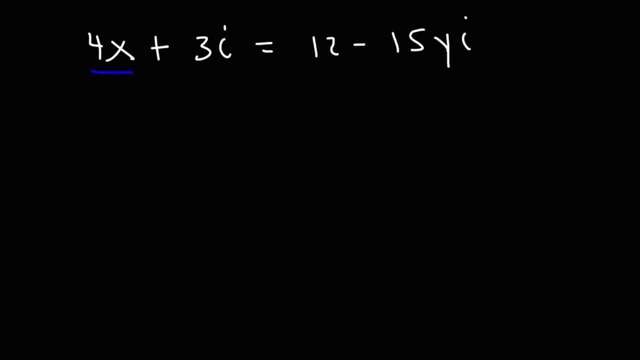 and the imaginary part. On the left side, 4x is the real part because it doesn't contain i. 12 is the real part as well, so we could set 4x equal to 12.. On the left side of the equation, 3i is the imaginary part, and so is negative 15yi. 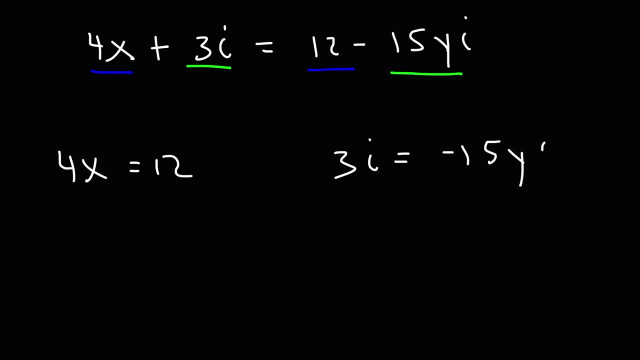 So we could set those two equal to each other. On the left we get that x is equal to 12 divided by 4, or 3.. And on the right, to isolate y, we need to divide both sides by negative 15i. 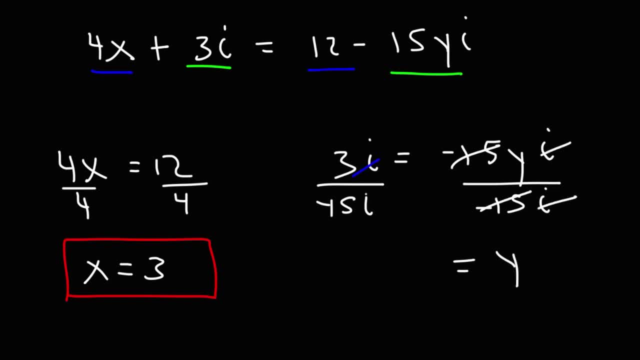 So we can cancel i And 3 over 15, if you divide both numbers by 3, you can reduce it to negative 1 over 5.. So that is the value of y in this equation. So that's how you can solve it. 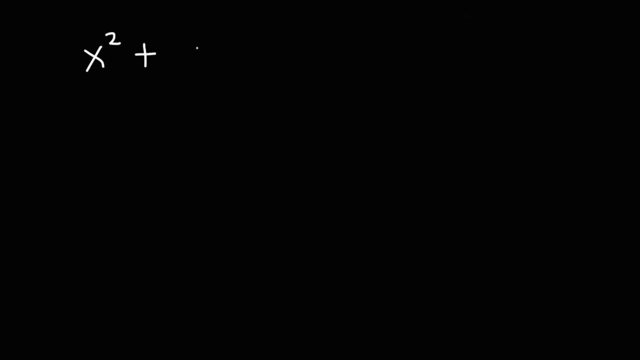 Now let's say, if we want to solve an algebraic equation like this one, Let's say that x squared plus 36 is equal to 0.. What is the value of x If you subtract both sides by 36.. 36.. 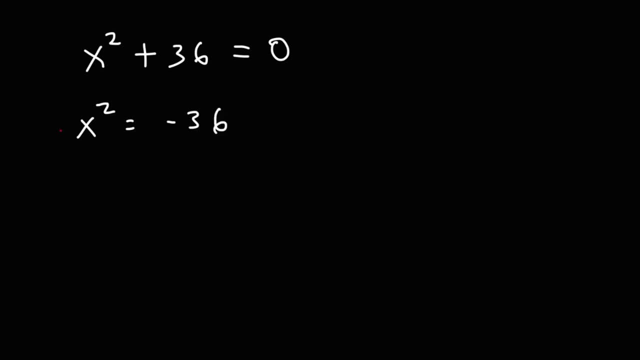 36., 36., 36., 36., 36.. get that x squared is equal to negative 36.. And if you take the square root of both sides, you realize that the solution is not a real answer. It involves imaginary numbers. So what? 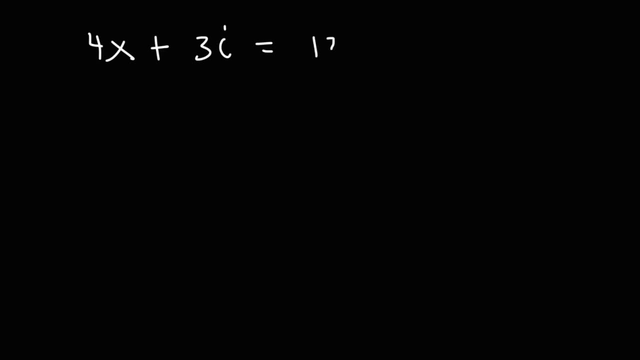 So let's say we have the equation: 4x plus 3i is equal to 12 minus 15y times i. So what is the value of x and y in this equation? In order to solve this equation, we need to identify the real portion of the complex number and the imaginary part. 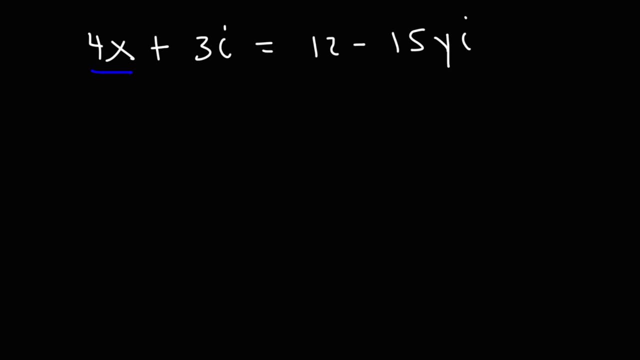 On the left side, 4x is the real part because it doesn't contain i. 12 is the real part as well, So we could set 4x equal to 12.. On the left side of the equation, 3i is the imaginary part, and so is negative 15yi. 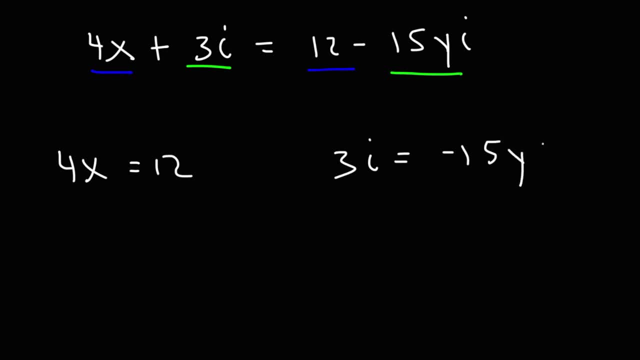 So we could set those two equal to each other. On the left we get that x is equal to 12 divided by 4, or 3.. And on the right, to isolate y, we need to divide both sides by negative 15i. 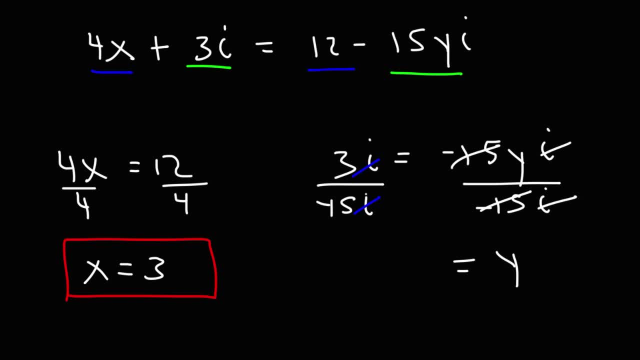 So we can cancel i And 3 over 15 is negative 15i. If you divide both numbers by 3,, you can reduce it to negative 1 over 5.. And so that is the value of y in this equation. 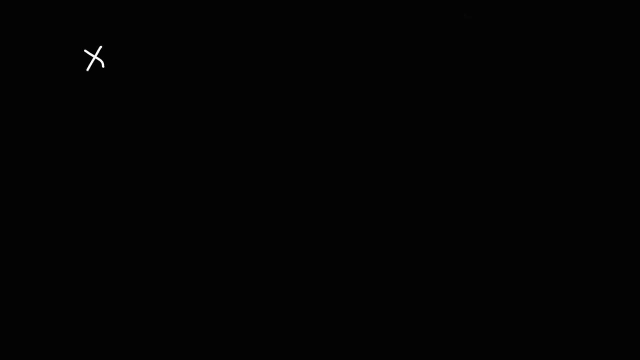 So that's how you can solve it. Now let's say: if we want to solve an algebraic equation like this one, Let's say that x squared plus 36 is equal to 0.. What is the value of x? If you subtract both sides by 36, you'll get that x squared is equal to negative 36.. 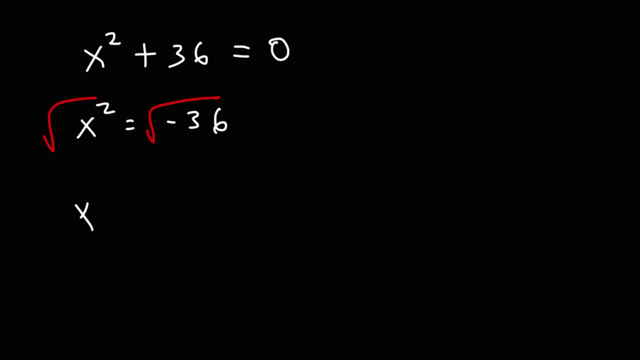 And if you take the square root of both sides, you'll realize that the solution is not a real answer. It involves imaginary numbers. So what is the square root of negative 36?? Well, we can write the square root of negative 36 as: 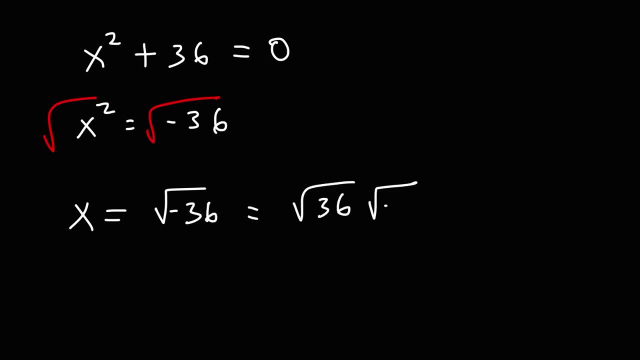 the square root of positive 36 times the square root of negative 1.. The square root of positive 36 is 6.. The square root of negative 1 is i, So we get this answer 6i, By the way, the square root of 36,. 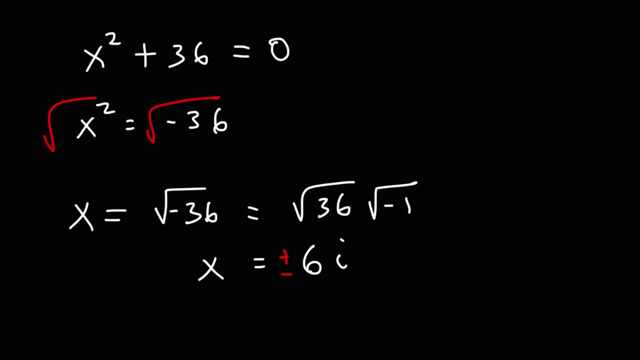 we can think of it as plus or minus 6.. Because we do get two solutions here, 6i and negative 6i, And we can test it out to make sure it works, For instance if we plug in 6i into the equation. 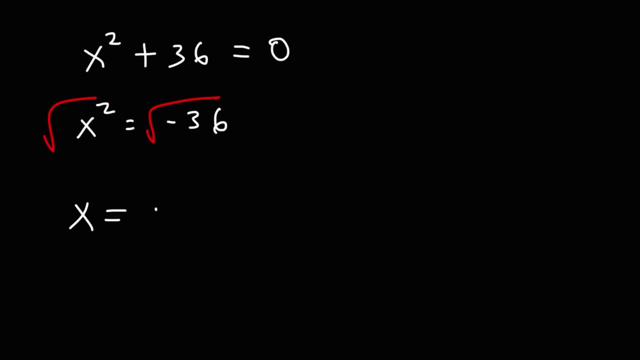 is the square root of negative 36?? Well, we can write the square root of negative 36 as the square root of positive 36 times the square root of negative 1.. The square root of positive 36 is 6.. The square root of negative 1 is i. 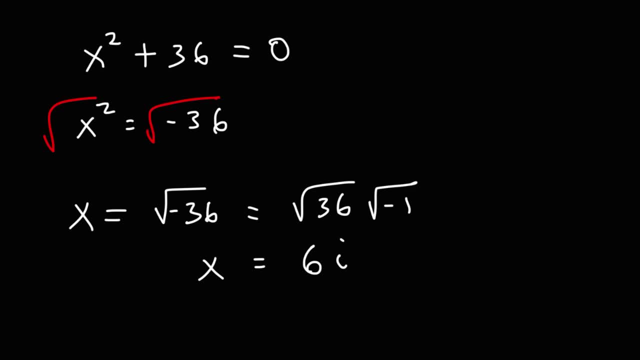 So we get this answer: 6i. By the way, the square root of 36, you can think of it as plus or minus 6, because we do get two solutions here, 6i and negative 6i, And we could test it out to make. 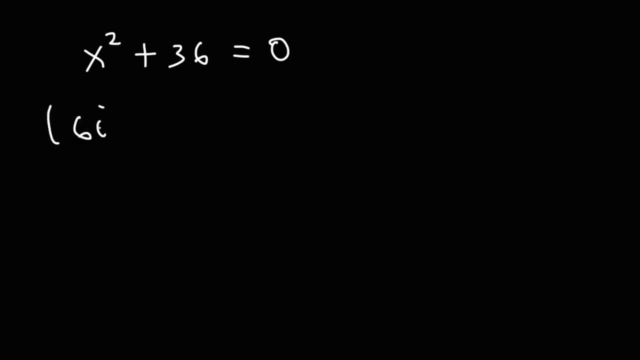 sure it works. For instance, if we plug in 6i into the equation, let's see if it gives us 0.. 6 squared is 36.. i squared is just i squared. Now we know that i squared is negative 1.. 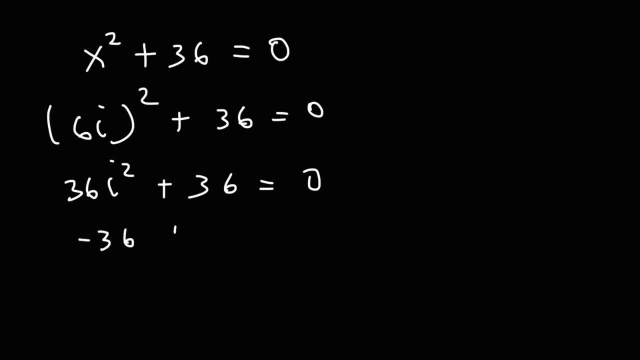 So we have 36 times negative 1. Which is negative 36. And so we get: 0 is equal to 0. This works. Now, if we were to try negative 6i, we would also get the same solution, because negative 6 times negative 6 is still. 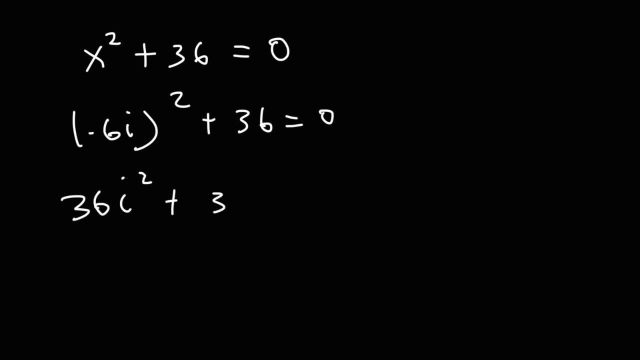 positive 36. And we're still going to get i squared as well. So the end result is still the same. Thus, the solution in this problem is: x is plus or minus 6i. Now let's work on one more example. Let's plot the complex number 4 plus 3i. 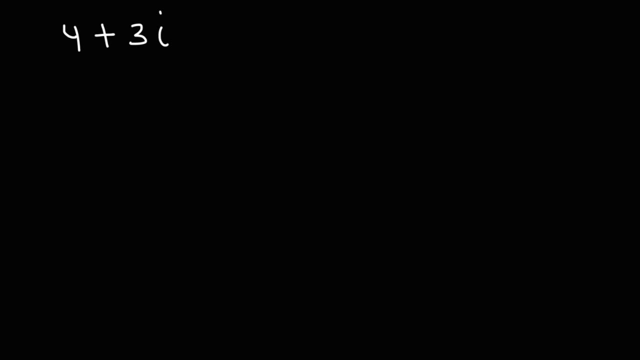 And at the same time let's calculate the absolute value of 4 plus 3i. So let's start with the absolute value. So the absolute value of a complex number in standard form is equal to the square root of 3i. 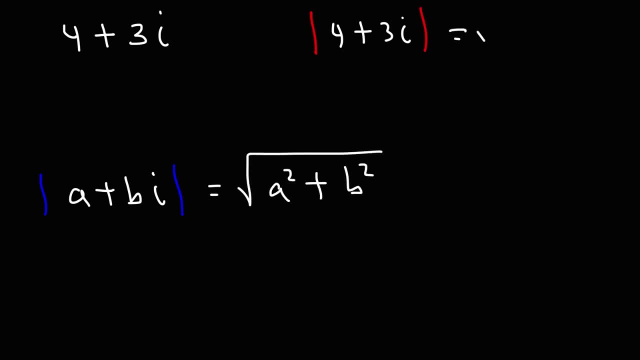 The absolute value of a square plus b squared. So in this case it's going to be the square root of 4 squared plus 3 squared. 4 squared is 16.. 3 squared is 9.. 16 plus 9 is 25.. 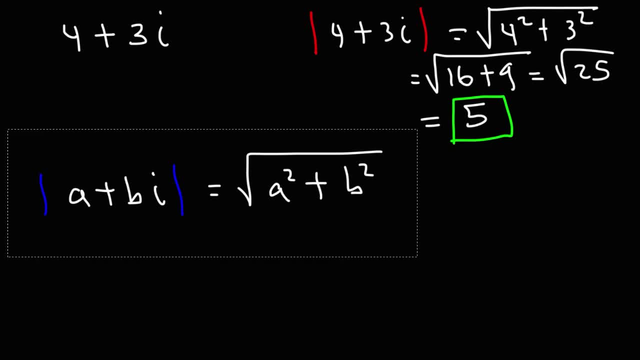 So the absolute value is going to be 5.. Now let's talk about how we can plot imaginary numbers. The x-axis is going to be the real axis, The y-axis is the negative x. So again, let's try to że a complex number of 1i. 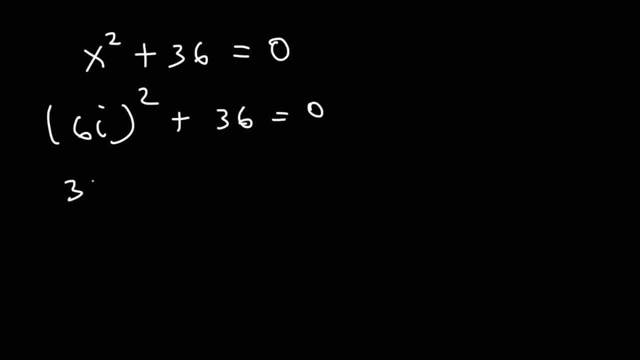 let's see if it gives us 0.. 6 squared is 36, i squared is just i squared. Now we know that i squared is negative 1.. So we have 36 times negative 1, which is negative 36.. 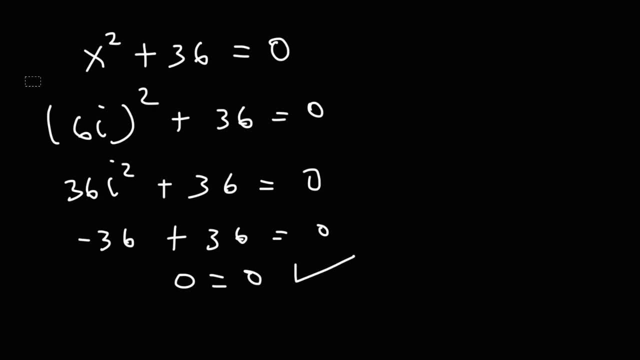 And so we get: 0 is equal to 0. This works. Now, if we were to try negative 6i, we would also get the same solution, Because negative 6 times negative 6 is still positive 36. And we're still going to get i squared as well. 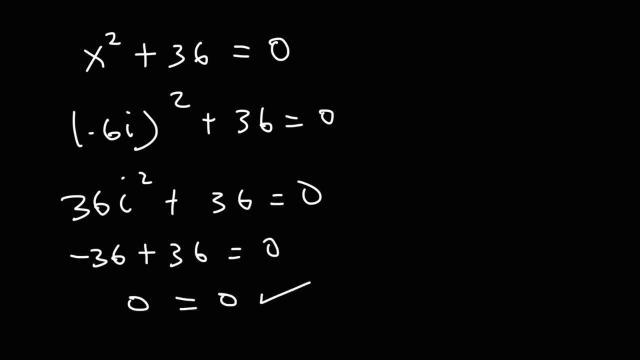 So the end result is still the same. Thus, the solution in this problem is: x is plus or minus 6i. Now let's work on one more example. Let's plot the complex number 4 plus 3i And at the same time let's calculate the absolute value of 4 plus 3i. 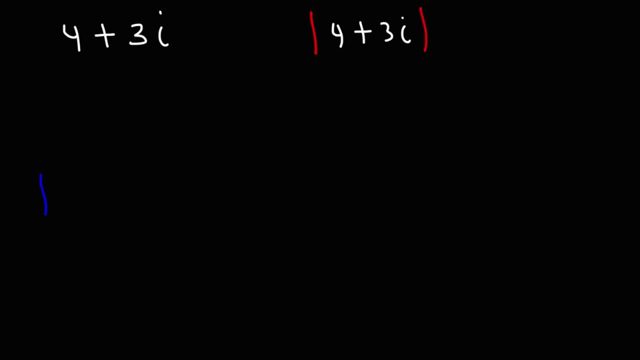 So let's start with the absolute value. So the absolute value of a complex number in standard form is equal to the square root of a squared plus b squared. So in this case it's going to be the square root of 4 squared. 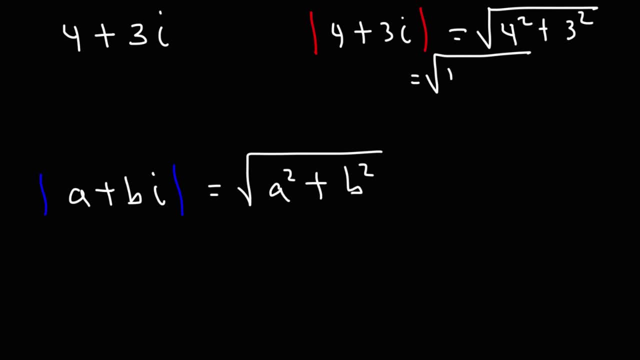 Plus 3 squared, 4 squared is 16.. 3 squared is 9.. 16 plus 9 is 25.. So the absolute value is going to be 5.. Now let's talk about how we can plot imaginary numbers. 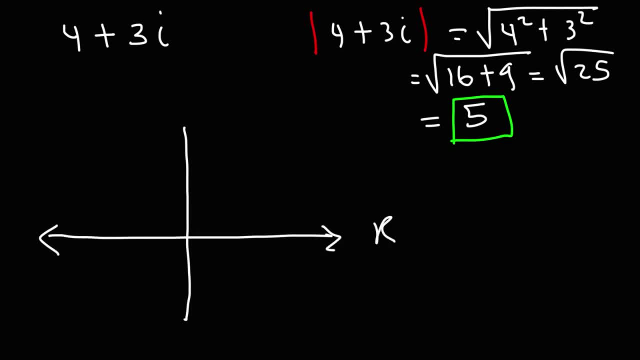 The x-axis is going to be the real axis. The y-axis will be the imaginary axis. So the real axis is going to be the imaginary axis. real number is 4.. So we're going to travel 4 units to the right. Now the imaginary number. 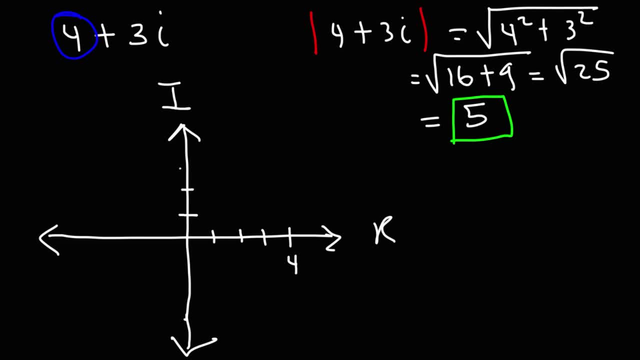 combined is 3i, So we're going to travel up 3 along the x-axis. So the point is located here. We traveled 4 units to the right and then up 3 units. The hypotenuse of this triangle represents the absolute value of the complex number, And so this is 5.. Thus what we have here.